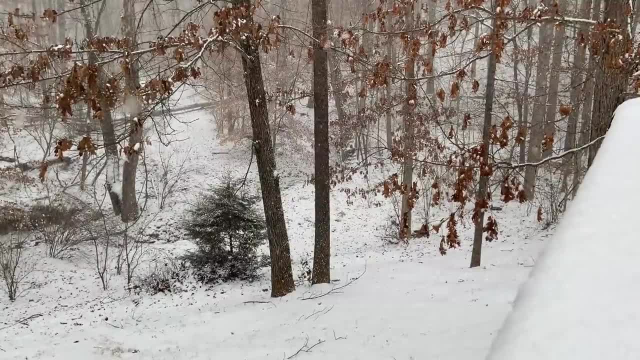 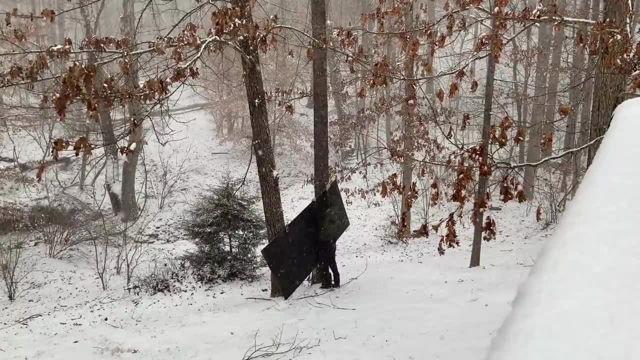 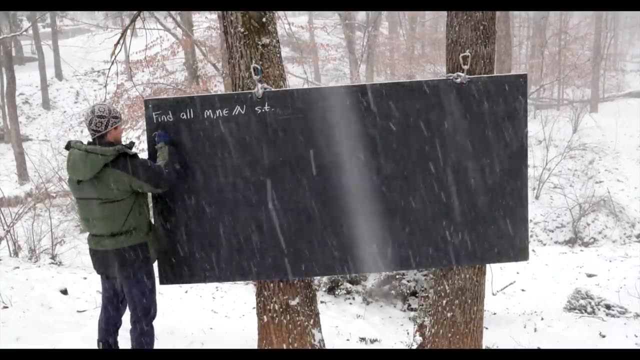 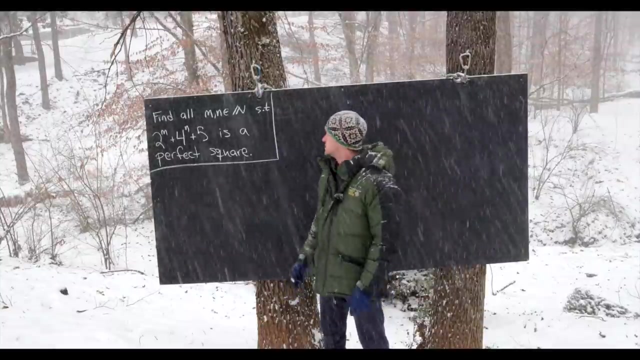 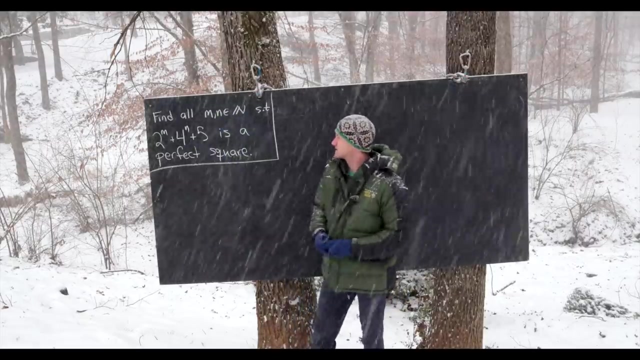 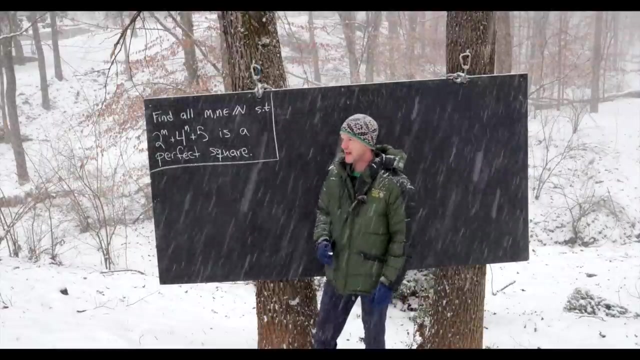 Here we're going to look at a nice quick number theory problem. So our goal is to find all natural numbers, m and n, such that 2 to the m plus 4 to the n plus 5 is a perfect square, And we're going to start by reducing modulo 8.. Why mod 8?? Well, that's because if n is bigger, 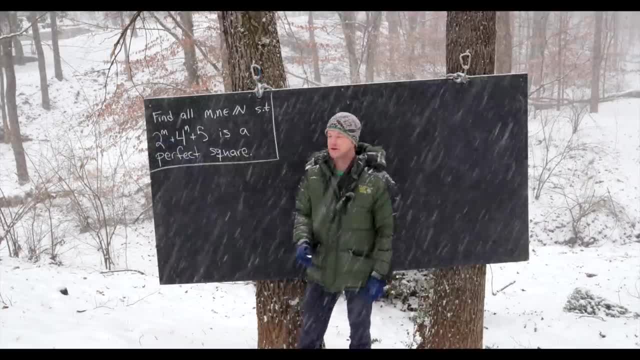 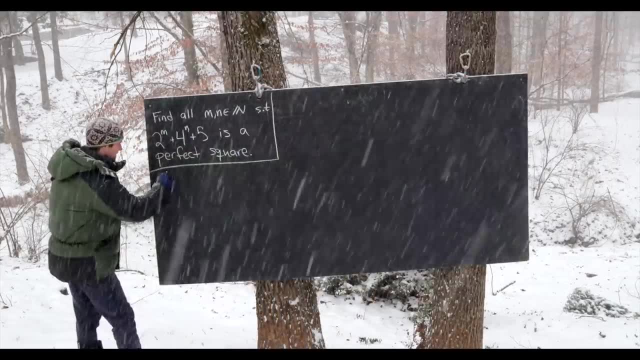 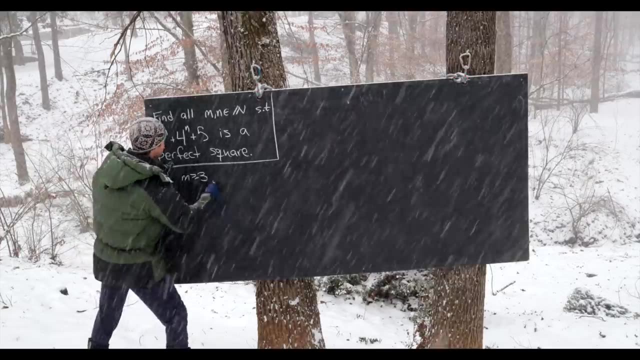 than or equal to 2 and m is bigger than or equal to 3,, these two guys reduce to 0 mod 8.. So let's point that out. So if, like I said, m is bigger than or equal to 3, then 2 to the m is a multiple of 8.. And if n is bigger than or equal, 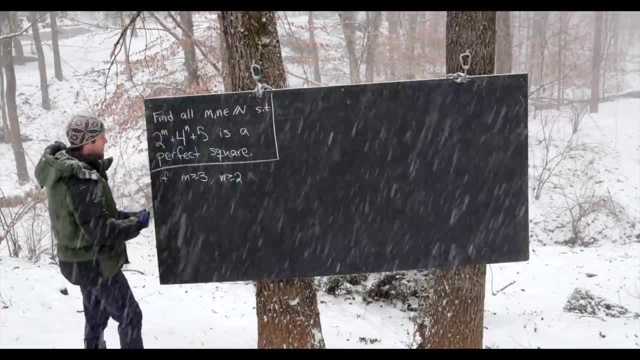 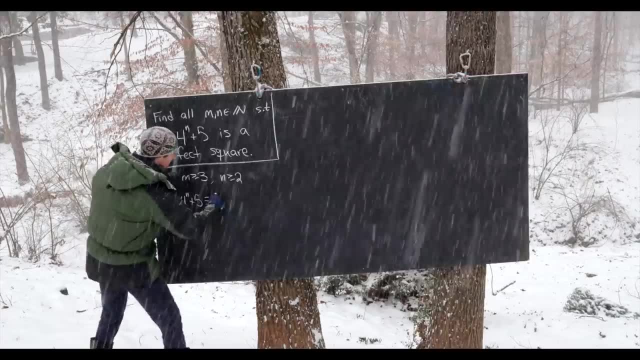 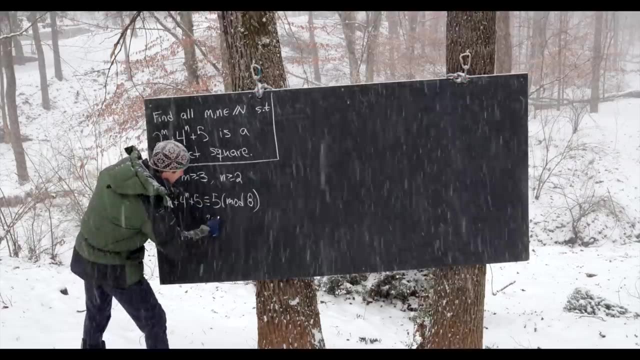 to 2, then 4 to the n is a multiple of 8.. So we have our object: 2 to the m plus 4 to the n, plus 5 will be congruent to 5 mod 8.. But 5 is not a square mod 8.. 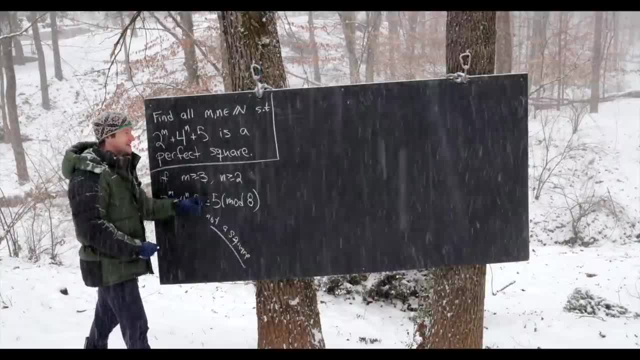 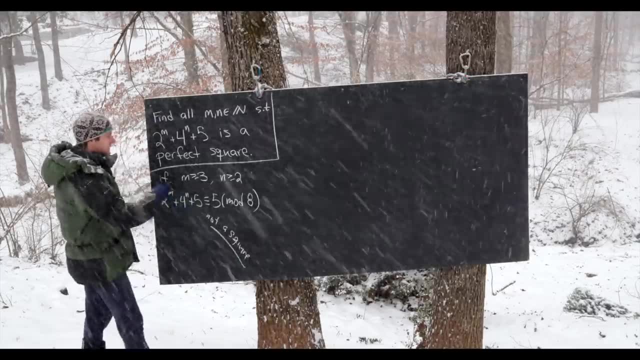 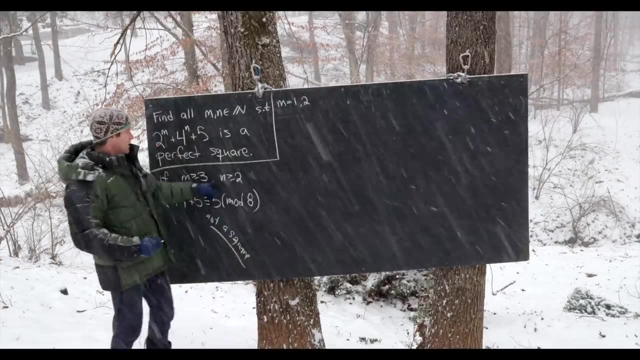 You can calculate that just by squaring everything mod 8 and see that it's impossible to achieve the number 5.. Well, so that tells us that the only possibilities for m are 1 and 2.. So m equals 1 or 2.. And the only possibilities for n are just 1.. So n equals 1.. So maybe 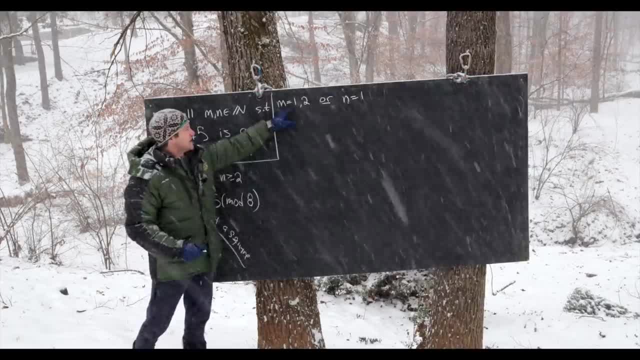 let's put an or here, Because just because m is 1 or 2,, that doesn't mean that n can only be 1.. So let's put an or here. So let's put an or here. So let's put an, or here, So. 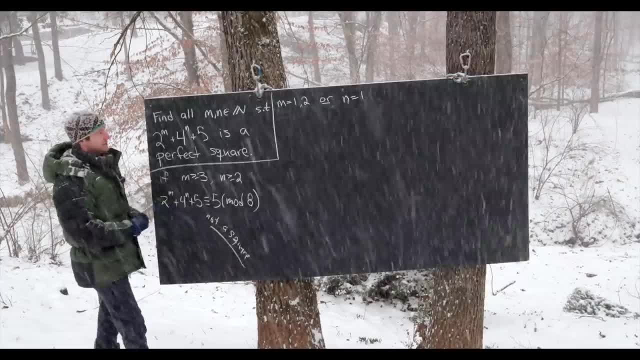 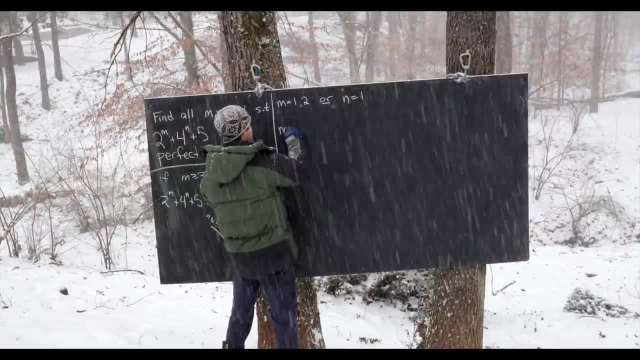 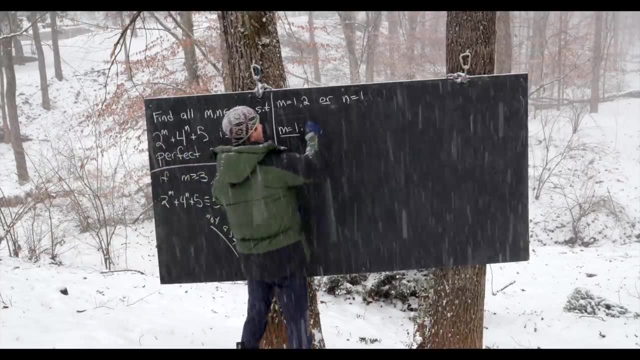 let's put an 1.. That's because this trick here relied on both of these reducing Okay. so now let's look at each of these cases on their own. So let's look at the case when m is equal to 1.. So let's notice: if m is equal to 1, we have 4 to the n, plus 7 must be a. 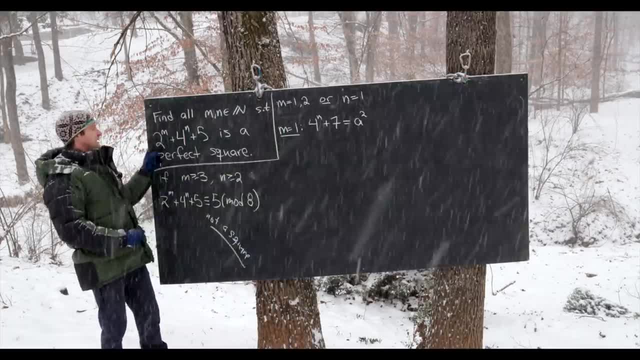 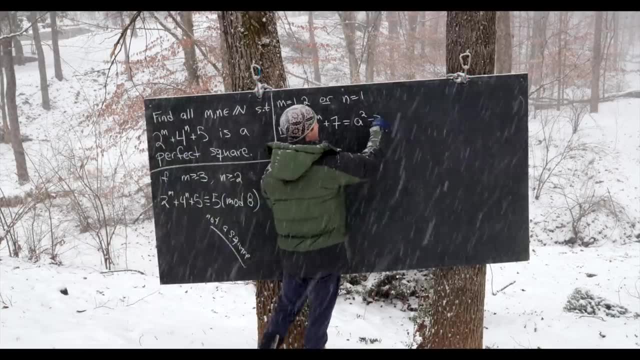 perfect square. I'll call it a squared. That's because we have: 2 plus 5 is 7.. But now we're we're going to reduce this mod 3 and we'll reduce this mod 3, because this is 1 mod 3 and this is. 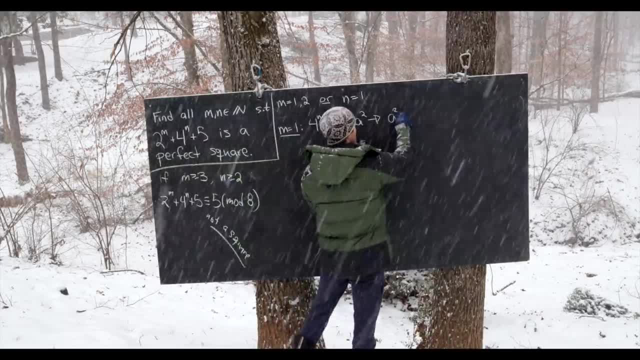 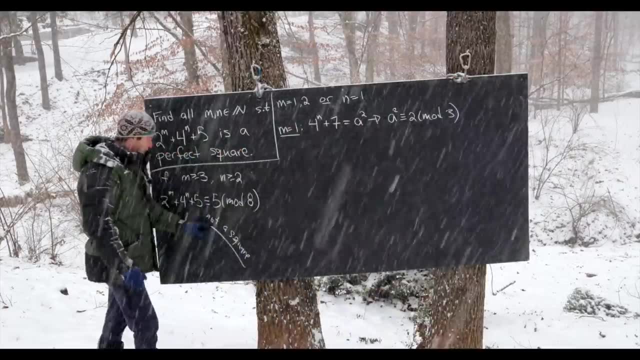 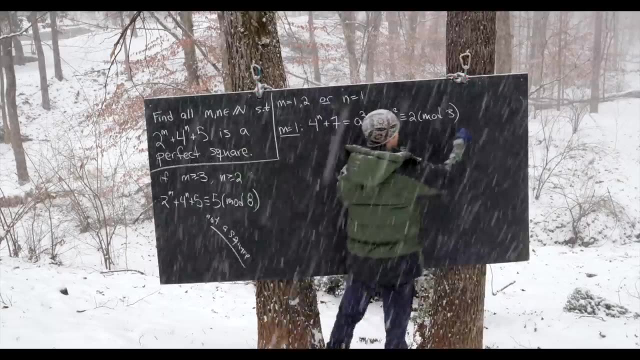 also 1 mod 3, telling us that we have a squared is 1 plus 1 or 2 modulo 3.. But just like over here, where we use the fact that 5 is not a perfect square mod 8, we also know that 2 is not a perfect. 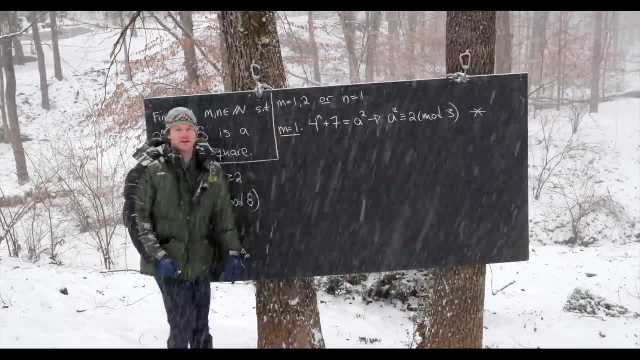 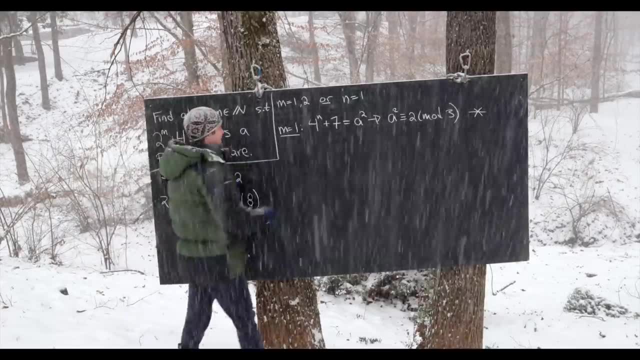 square mod 3.. The only squares mod 3 are 0 and 1.. So that means we do not get a solution in this case when m is equal to 1.. So now let's move on to the case when m is equal to 2. 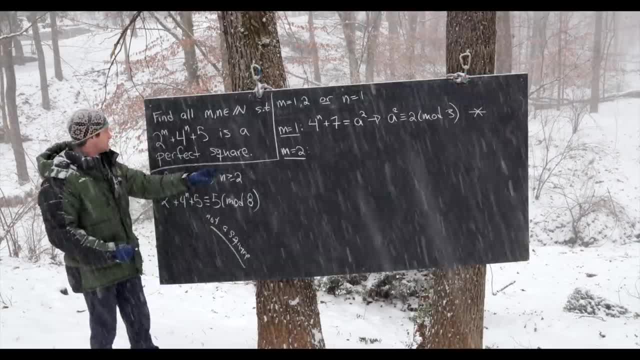 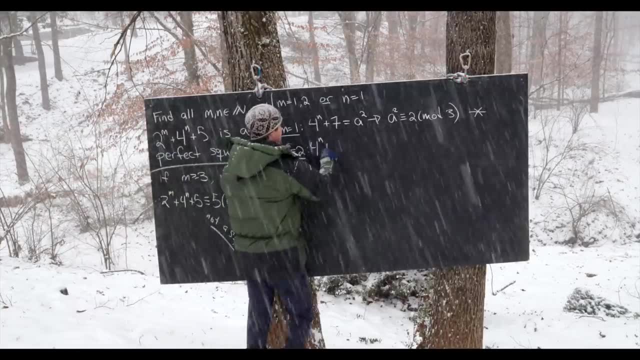 and see what happens. So if m is equal to 2, we have 2 squared, plus 5 is 9.. So that means we have 4 to the n plus 9 is a perfect square like that. But let's notice that we. 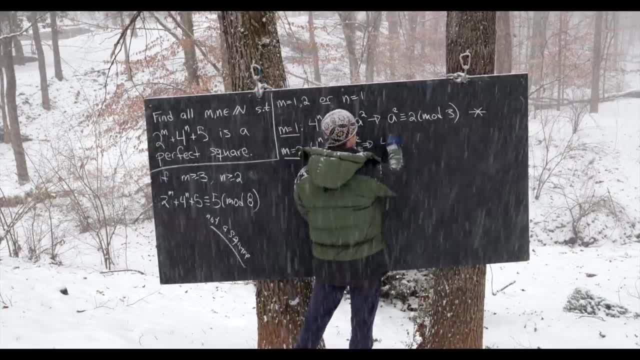 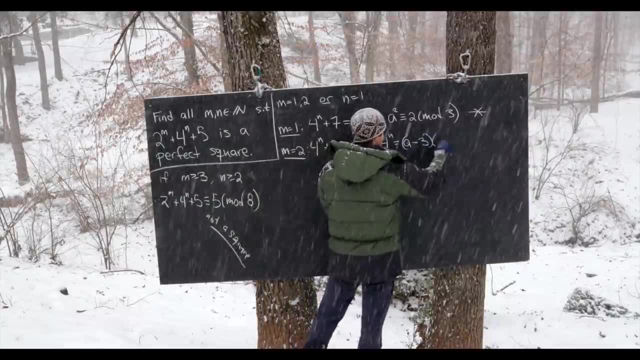 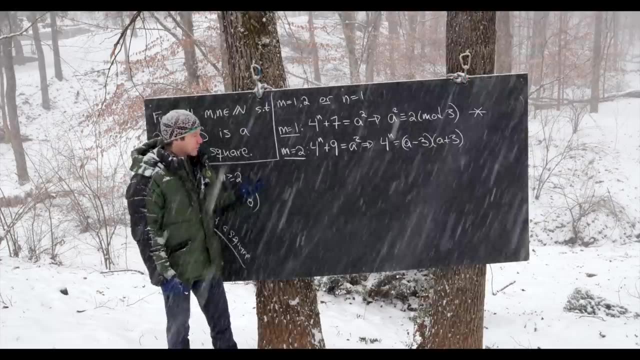 can reduce this really quickly to: 4 to the n is equal to a squared minus 9, which we can factor as a minus 3 times a plus 3.. But now let's notice that 4 to the n is a power of 2. That means the 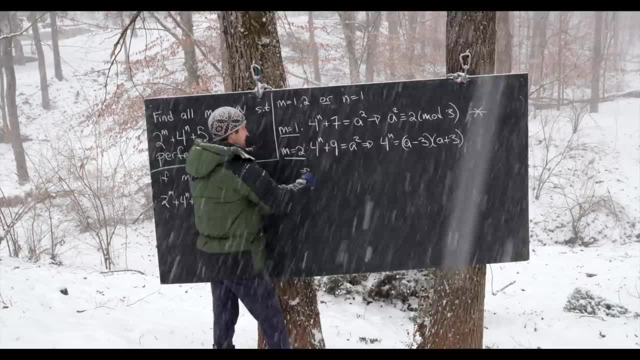 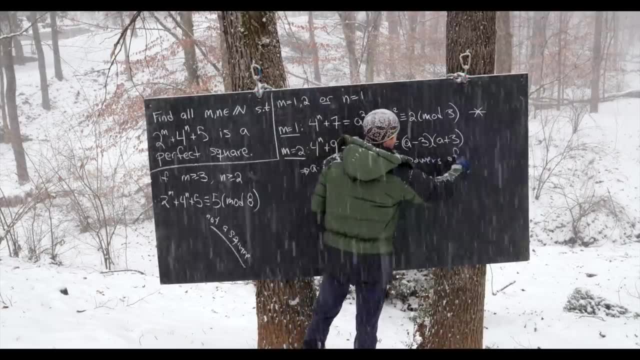 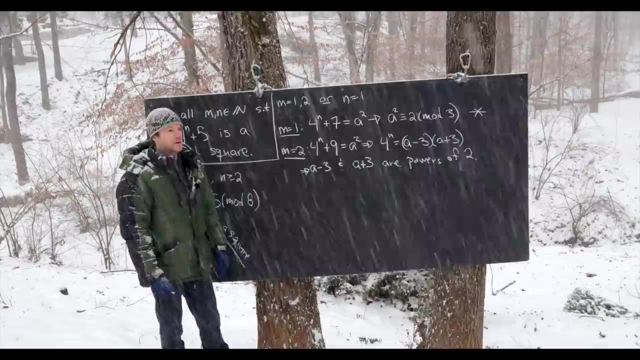 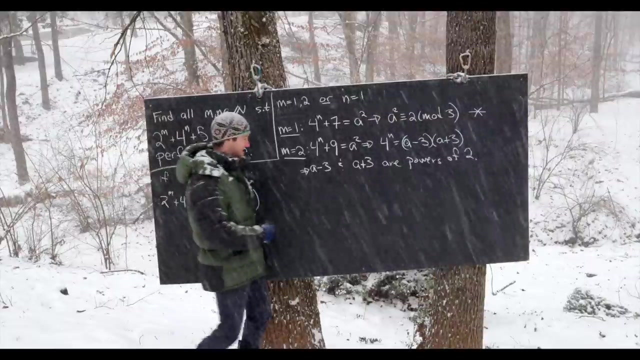 right hand side is also a power of 2.. In particular, a minus 3 and a plus 3 are powers of 2.. Furthermore, there are powers of 2 that differ by 6.. But there are only two different powers of 2 that differ by 6, and that's the number 2 and the number 8. So that means a minus 3 is 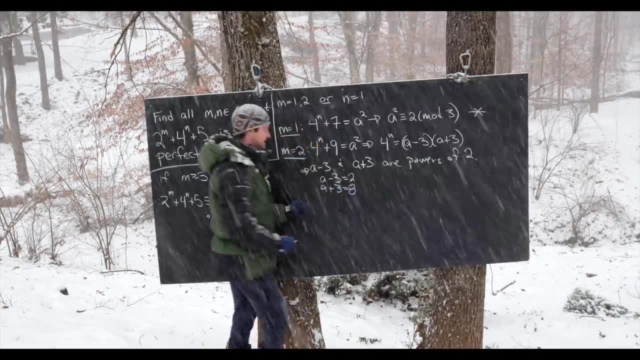 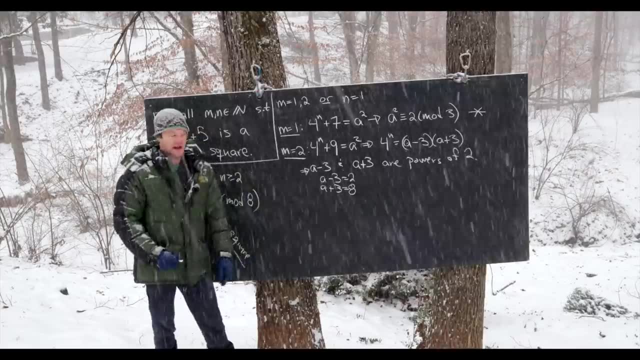 equal to 2 and a plus 3 is equal to 8.. Like I said, those are the only two powers of 2 that differ by 6.. We know they differ by 6, because a minus 3 to a plus 3.. Okay, so now. 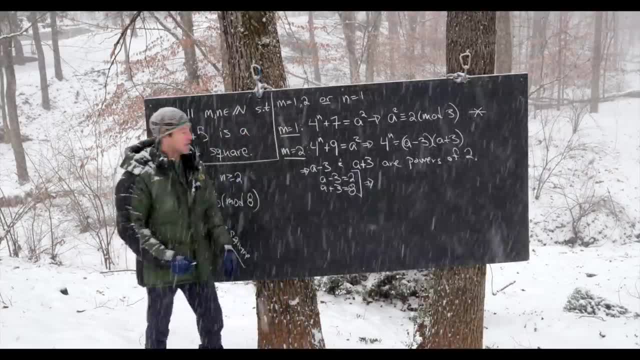 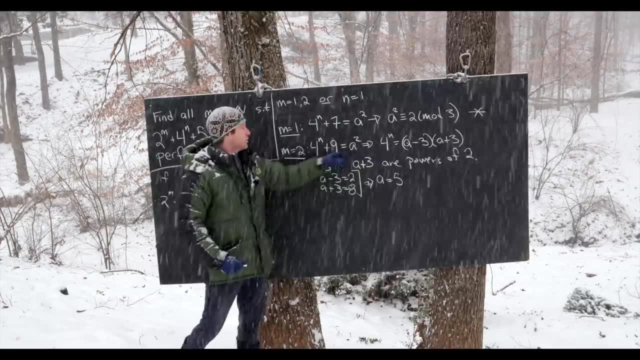 smushing this together. well, actually we can only solve one of them. if you'd like, We'll get that. a is equal to 5.. But now, plugging that back in up here, we see that 4 to the n is 25 minus 9..